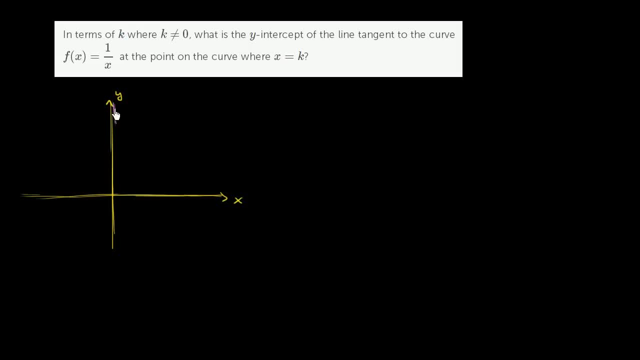 So it looks something like this. So it kind of spikes up there and then it comes down and then it goes like this- And I'm just doing a rough approximation of it, so it looks something like that. And on the negative side it looks something like this: 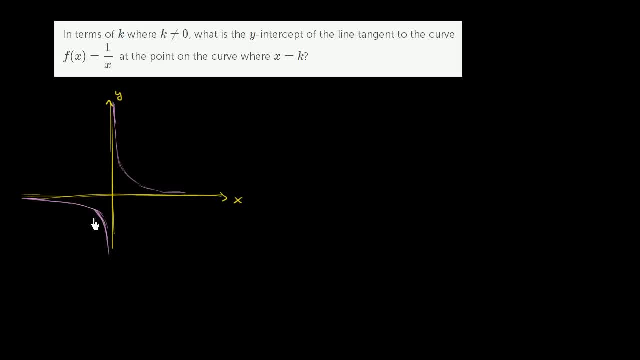 So this is my hand-drawn version of roughly what this graph looks like. So this right over here is f of x is equal to 1 over x. Now we are concerning ourselves with the point x equals k. So let's say, I mean, it could be anything that's non-zero. 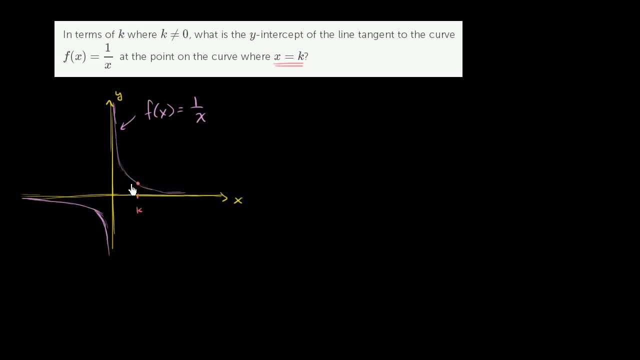 but let's just say that this is k right over here. So that is the point: k, 1 over k. We can visualize the line tangent to the curve there, So it might look something like this And we need to figure out its y-intercept. 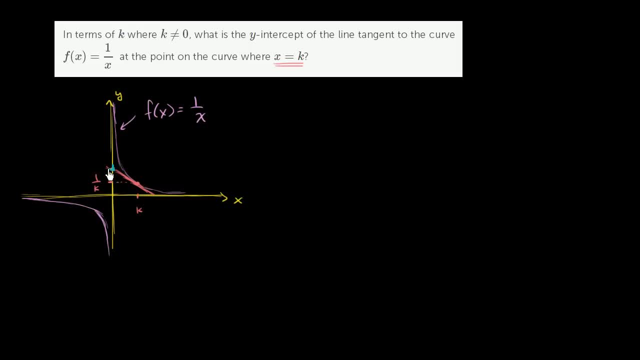 How does it intercept the y-axis? So we need to figure out this point right over here. Well, the best way to do it if we can figure out the slope of the tangent line. here, the slope of the tangent line is just the derivative. 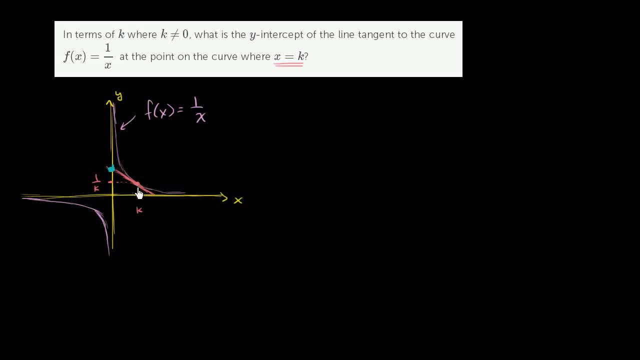 of the line at that point, If we could figure out the slope of the tangent line. we already know that that line contains the point. We already know it contains the point, This point right over. let me do this in a different color. 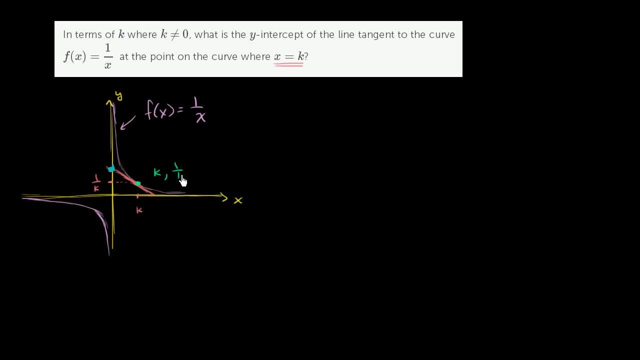 We know it contains the point k, comma 1, over k. So if we know its slope, we know what point it contains, we can figure out what its y-intercept is. So the first step is: well, what's the slope of the tangent line? 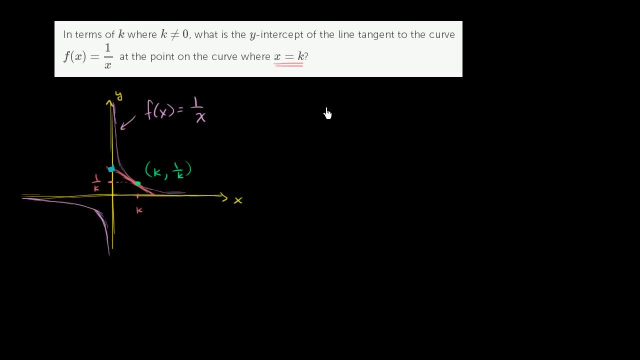 Well, to figure out the slope of the tangent line, let's take the derivative. So if we write f of x, instead of writing it as 1 over x, I'll write it as x to the negative 1 power. that makes it a little bit more obvious. 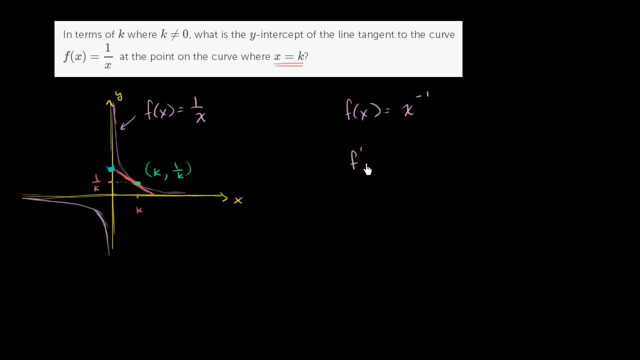 that we're about to use the power rule here. So the derivative of f at any point x is going to be equal to Well, the exponent here is negative one. so negative one times x to the. now we decrement the exponent to the negative two power. 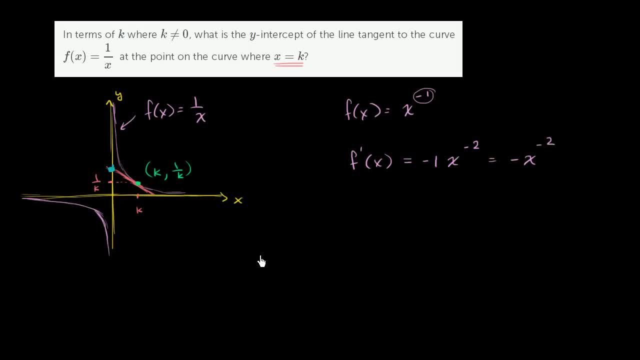 Or I could say it's negative x to the negative two. Now what we care about is the slope when x equals k, So f prime, f prime of k is going to be equal to, is going to be equal to negative k to the negative two power to the negative two power. 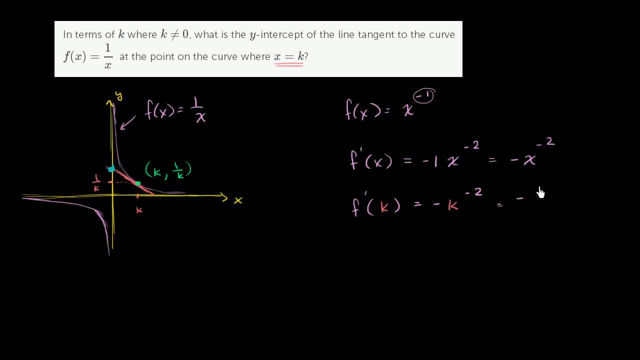 Or another way of thinking about it, this is equal to negative one over k squared, Negative one over k squared. So this, right over here, is the slope of the tangent line. at that point Now let's think about- well, let's just think about what the equation 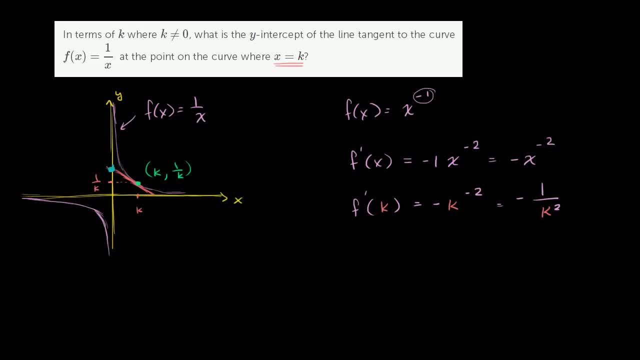 of the tangent line is: and we could think about it in slope intercept form. So we know the equation of a line in slope intercept form is: y is equal to mx plus b, where m is the slope and b is the y intercept. 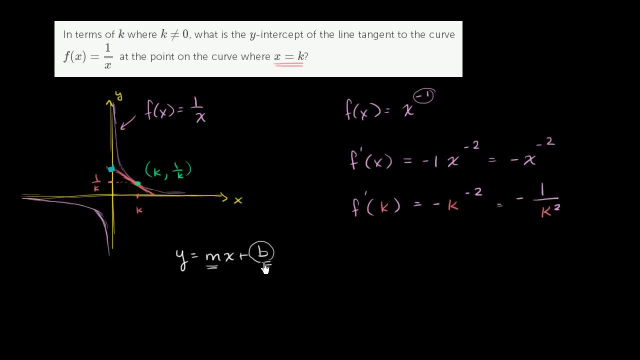 So if we can get it in this form, then we know our answer, We know what the y intercept is going to be. It's going to be b. So let's think about it a little bit, This equation. so we could say: y is equal to our m. 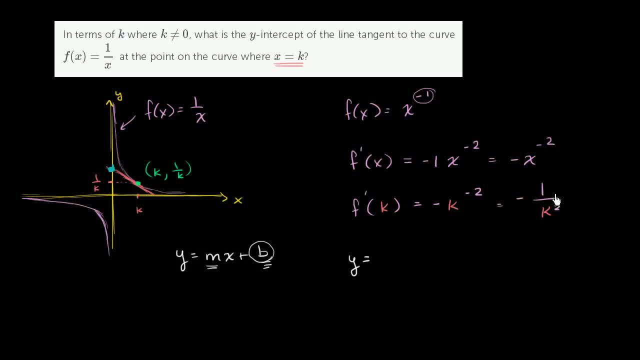 our slope of the tangent line. when x is equal to k, we just figure out to be this business, It equals this thing right over here. So let me write that in blue Negative one over k: squared times x, times x plus b. 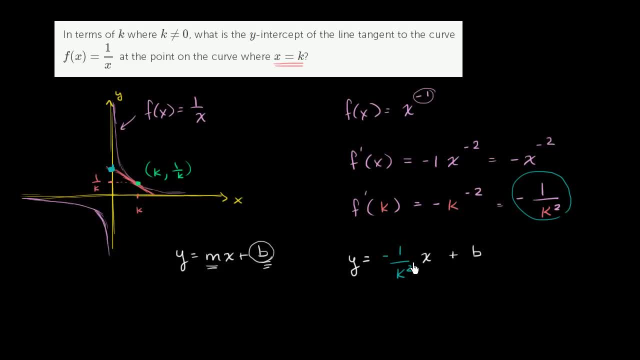 So how do we solve for b? Well, we know what y is when x is equal to k, and so we can use that to solve for b. We know that y is equal to one over k, y is equal to one over k. 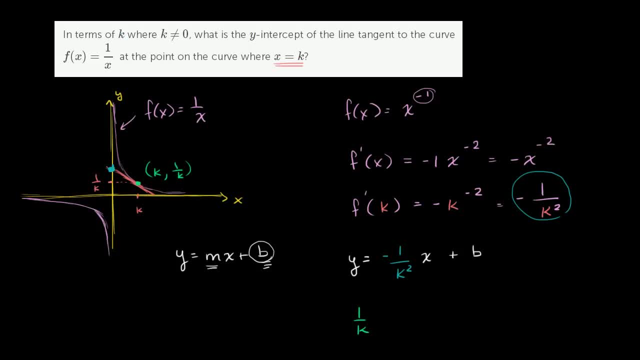 when x is equal to k, So this is going to be equal to. I'm gonna keep the colors consistent: equal to negative one that's not the same color, negative negative one over k. squared times k times k plus b plus b. 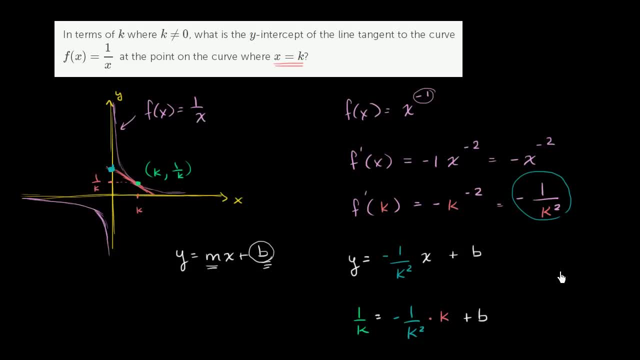 do that in white plus b. Now what does this simplify? to See k over k squared is the same thing as one over k. so this is going to be negative one over k. So this part, all of this, all of this simplifies to negative one over k.